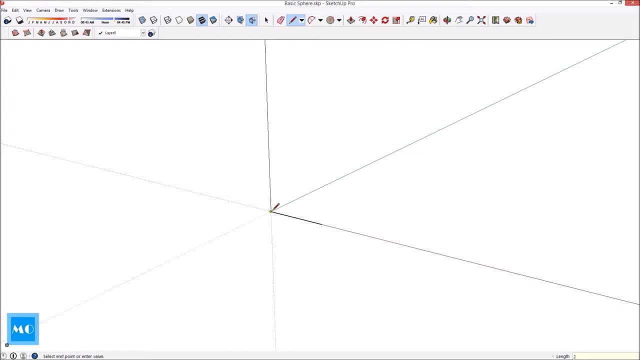 The second line starts at the origin and extends 2 meters in the negative X direction. Our third line starts from the end point of the first line. It extends 3 meters in the positive X direction. We repeat the process and draw another 2 lines, each 3 meters in length, along the positive X direction. 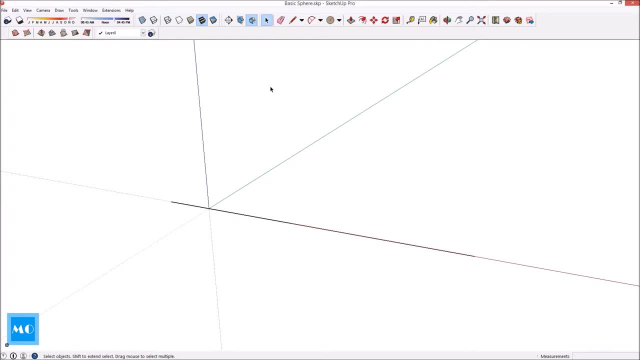 We can now draw our circles using the guidelines we have created. The first circle starts at the origin and closes at the end point in the negative X direction. In this way, we create our first circle, which is 4.. The second circle starts at the end point, between the 4th and 5th lines, and closes at the last end point. 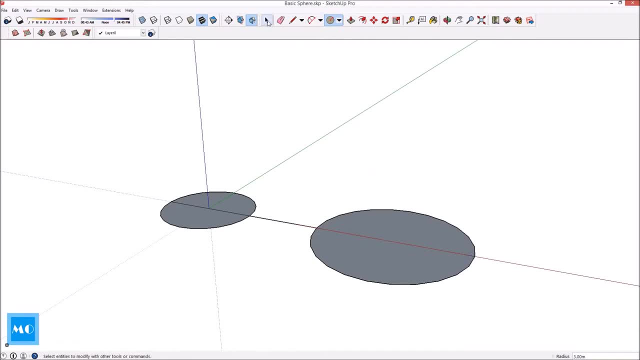 In this way we create the second circle, which is 6 meters in diameter and centered along the X axis. We can now delete the middle construction line which was used to separate our two circles. Next, we rotate the largest circle in the green direction, Left click and drag the mouse until the circle is separated. 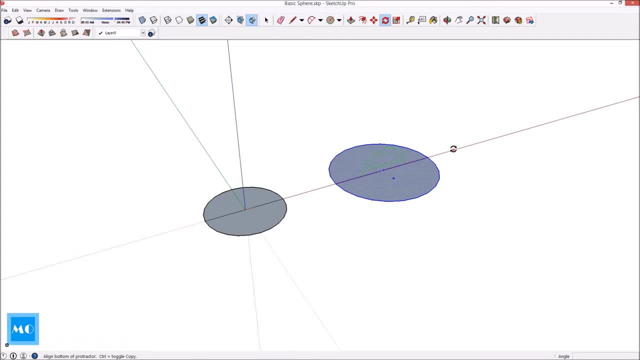 Before the green guide lock appears. we can then snap the guide to a 20 degree angle and rotate the circle. We now use the MOVE command to move the larger circle to be centered on top of the smaller circle. The circle center lock should be used to position the circles in place. 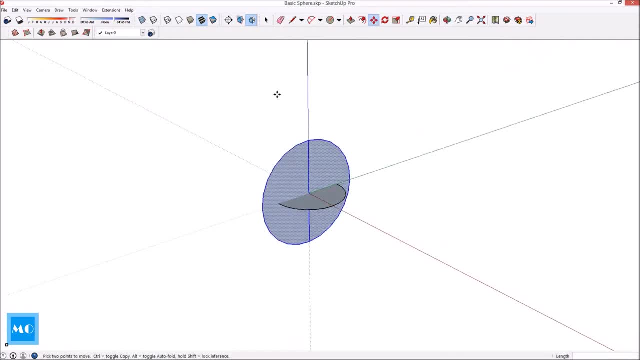 Oh my, this sucks. Goodbye. Our construction guidelines can now be deleted. This will leave us with a perimeter outline of the smallest circle and the closed surface of the larger circle. Select the perimeter outline of the smaller circle. Under the tools drop down, choose the follow me command. 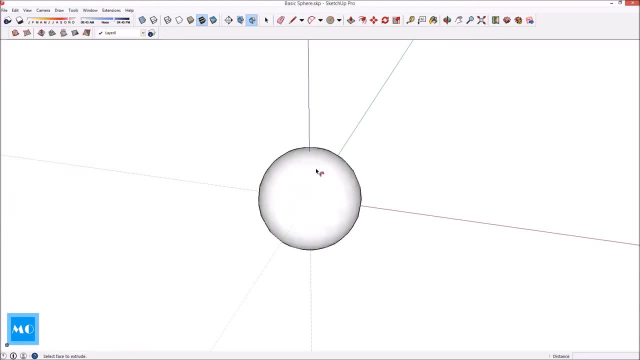 Next click on the surface of the larger circle. This should transform the 2D circle surface into a 3D spherical surface. The follow me command has extruded the circle surface around the smaller circle guideline. By triple clicking the 3D spherical surface, the individual segments of the sphere can